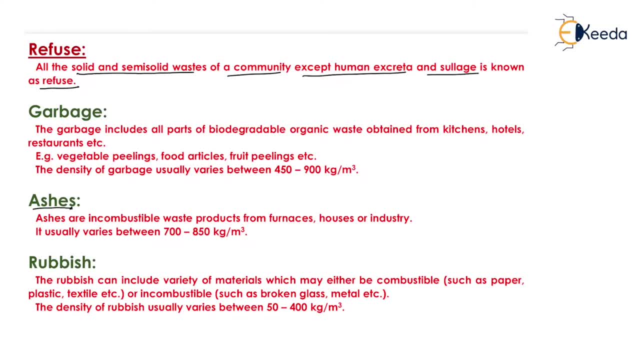 It means that all the solids and semi-solid waste of a particular community, except the human solid waste that is, excreta and slage, is known as refuse. Now, what are the examples of refuse? The examples of refuse are garbage ashes and rubbish. 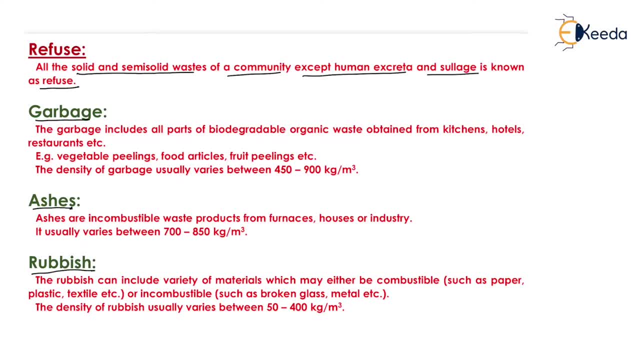 Now, what is garbage? Garbage includes all parts of biodegradable organic waste obtained from kitchen, hotels, restaurant, etc. It means that garbage will include all parts of organic waste obtained from kitchen, hotels, restaurant, etc. It means that garbage will include all parts of organic waste obtained from kitchen, hotels, restaurant, etc. 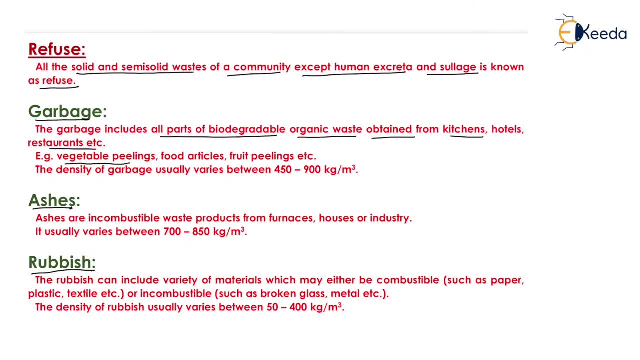 Now, what are the examples of garbage? Vegetable peelings, food articles, fruit peelings are the examples of garbage. Now, the density of garbage usually varies between 450 to 900 kg per meter cube. That is the garbage. Now what is ashes? Ashes are the incombustible waste product obtained from furnaces, houses or industries. 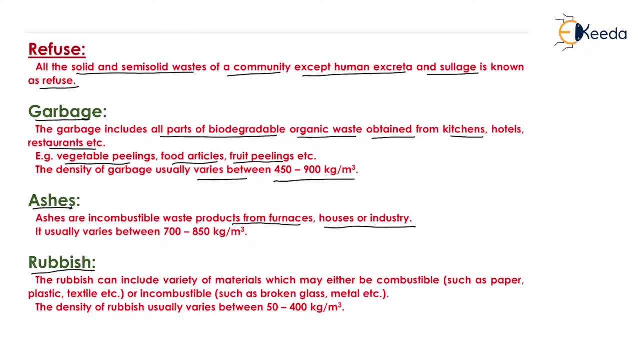 When we burn the solid waste in the large incinerators or furnaces, all the combustible material will evaporate or goes out into the atmosphere and all the incombustible material will remain in the furnaces itself in the form of ashes. When we burn the solid waste in the large incinerators or furnaces, all the combustible material will evaporate or goes out into the atmosphere and all the incombustible material will remain in the furnaces itself in the form of ashes. 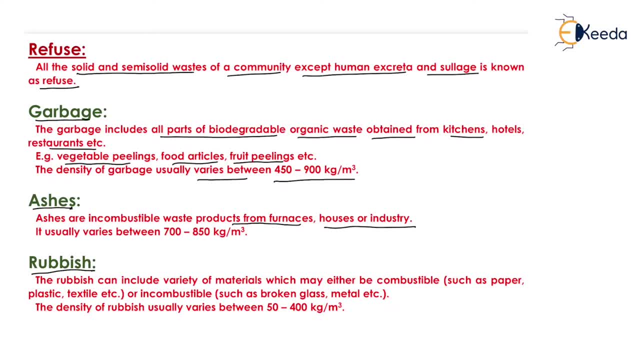 When we burn the solid waste in the large incinerators or furnaces, all the combustible material will evaporate or goes out into the atmosphere, and all the incombustible material will remain in the furnaces itself in the form of ashes. Now this ashes needs to be disposed by some other means. okay now. its density usually varies between 700 to 850 kg per meter cube. Now, what is rubbish? 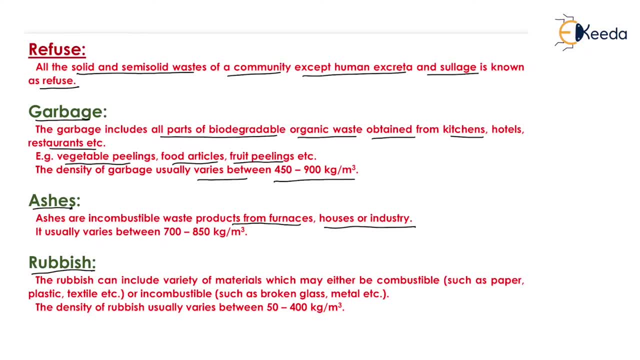 Now this ashes needs to be disposed by some other means. okay, now, its density usually varies between 700 to 850 kg per meter cube. Now, what is rubbish? Rubbish can include variety of materials which may either be combustible, such as paper, plastic, textiles, etc. or incombustible, such as broken glass, metal, etc. So we can say that rubbish is a combination of both combustible as well as incombustible material. 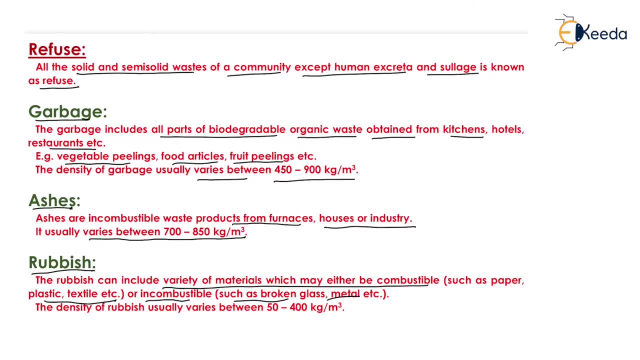 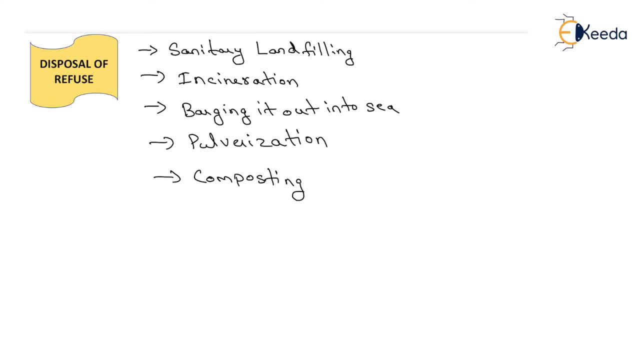 Now, the density of rubbish usually varies between 50 to 400 kg per meter cube. Now we will discuss the disposal of refuse. There are five methods of disposal of refuse. First one is the sanitary land filling, next one is the incineration, another one is barging it out into sea, next one is the pulverization and the last one is composting, which is the most important method of disposal of refuse. 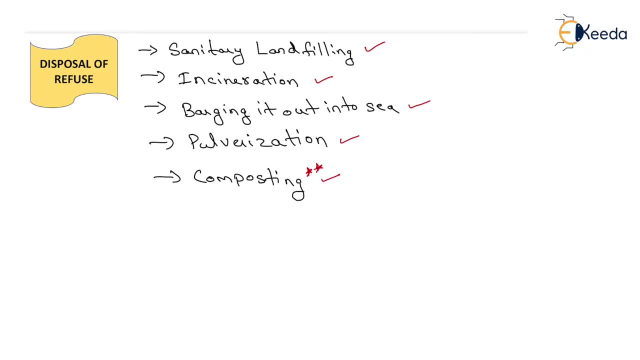 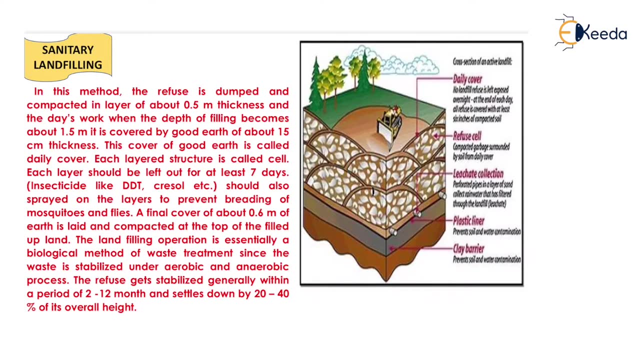 Now we will see each and every method in this video. Now we will see each and every method in detail, starting with the sanitary land filling. Now, what is sanitary land filling and how can it work? In this method, the refuse is dumped and compacted in layer of about 0.5 meter thickness, and the days work when the depth of filling becomes equals to 1.5 meter, it is covered by good earth of about 15 centimeter thickness. 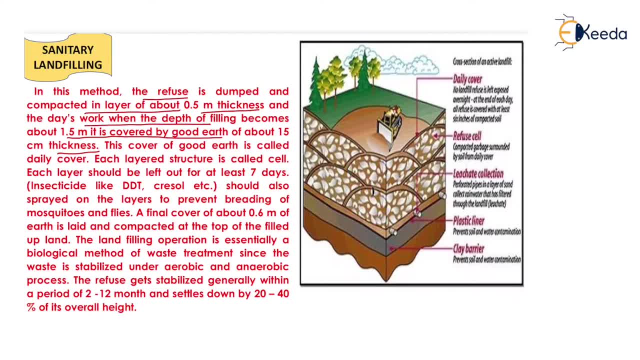 Now the land on which the sanitary land filling is to be done is covered with clay barrier so that land pollution will not happen on that land. Now, above that clay layer, perforated pipe should be provided so that all the liquid from the refuse will enter into this perforated pipe and from this perforated pipe we will take that liquid and dispose it by some other means. 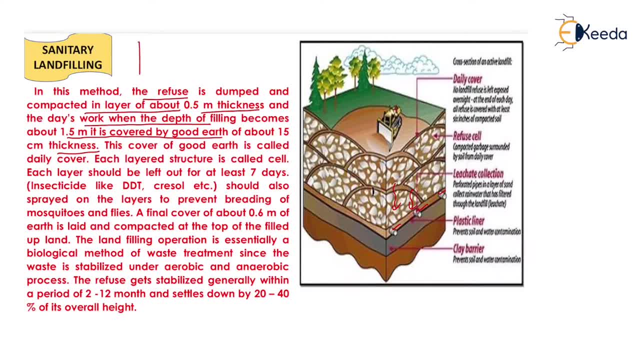 Now suppose that this is the plan of the area where we need to dispose or where we need to fill the land by sanitary land filling method. Now we divide this area into smaller units and this smaller unit is known as cell. Now we have to fill this smaller units one by one. Now we will show here the cross section of each cell. 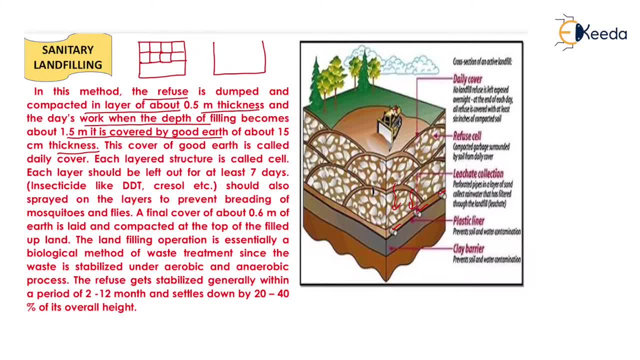 Now what will happen? Firstly, we will fill 0.5 meter thick refuse layer in this and compact it, After which we again add 0.5 meter of refuse and again compact it, and we will continue this till the height of 1.5 meter is not reached at the end of the days work. 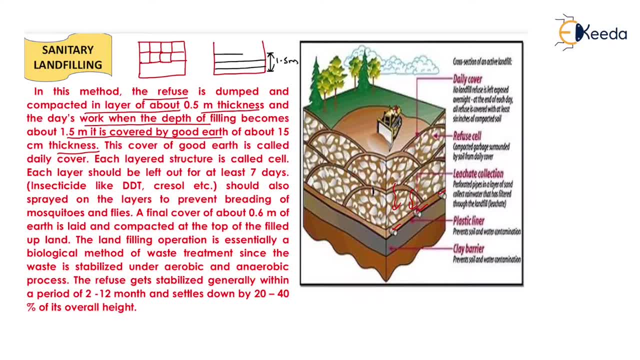 Now, when the height of 1.5 meter is not reached, at the end of the days, work is reached, we will cover this refuse by a 15 centimeter thick layer of soil. okay, now we will left this layer or we will left that cell for the seven days for its decomposition process. now, 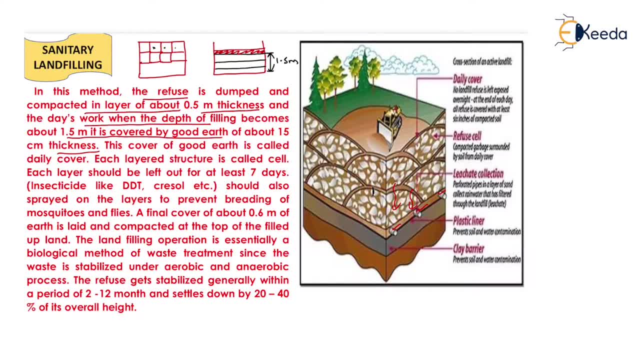 in the next day we will fill next cell. similarly, we will fill next cell in the next seven days. now, after seven days, we will again fill this same cell, again by 0.5 centimeter refuse, then by 0.5 meter refuse, then 0.5 meter refuse, till 1.5 meter height is not reached, after which 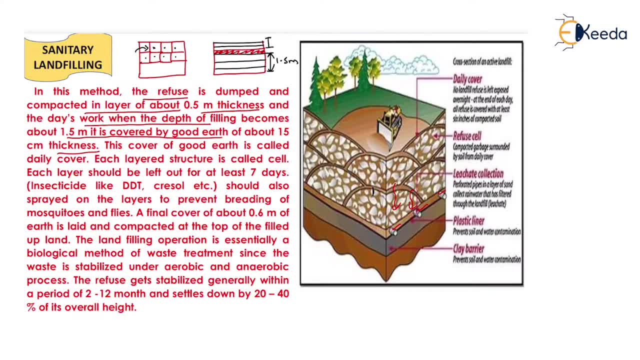 the process is same and repeated. okay, now, during this seven days, insecticides like ddt, cresol, etc. should be sprayed on it so as to prevent the breeding of mosquitoes and flies. when the land is completely filled by refuse, a final cover of about 0.6 meter of earth is laid and compacted at. 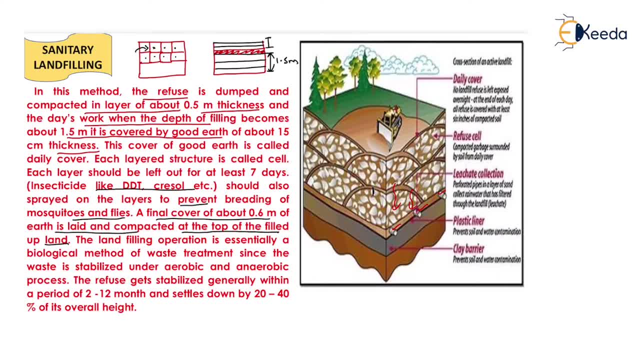 the top of the filled up land. okay, now, when the height, when the area is completely filled by refuse, we need to cover that refuse by 0.6 meter of earth. okay now, the land filling operation is essentially a biological method of waste treatment, since the waste is stabilized under aerobic condition. starting. 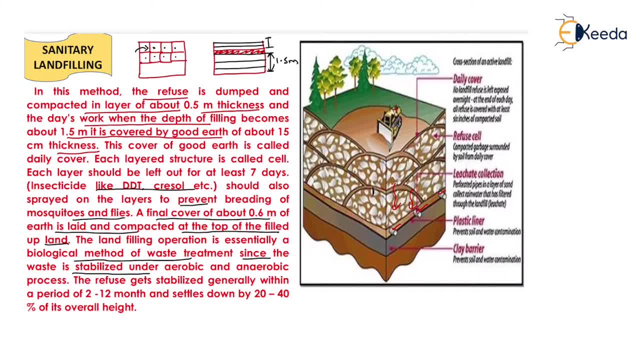 okay. during the starting of this process, the condition will be aerobic because oxygen is there. now. when the time goes, then the oxygen deficiency is there. okay. now. when the time goes, then the oxygen deficiency is there. okay now. when the time goes now, due to the deficiency of the oxygen, what will happen? an aerobic process will takes place in. 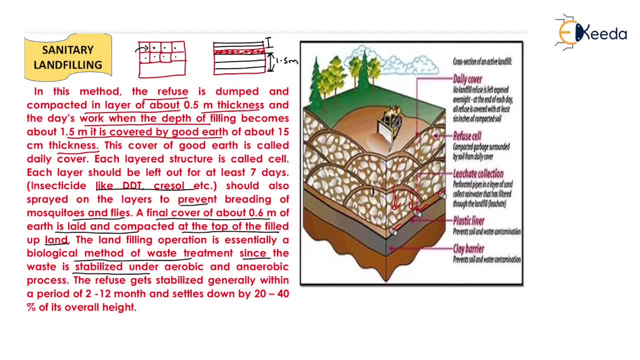 that sanitary land filling. okay, so we had right here. the waste is stabilized under aerobic and anaerobic processes. the refuse gets stabilized generally within the period of 2 to 12 months and settled down by 20 to 40 percent of its overall height. it means that the complete land 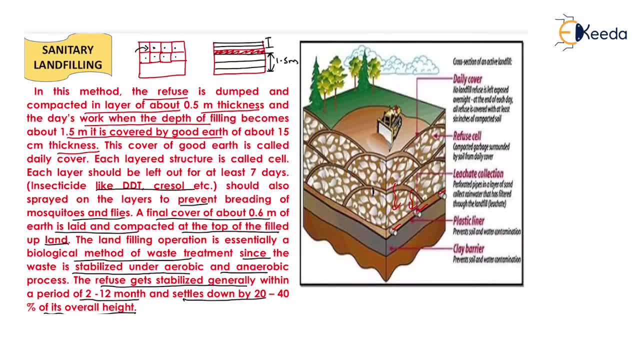 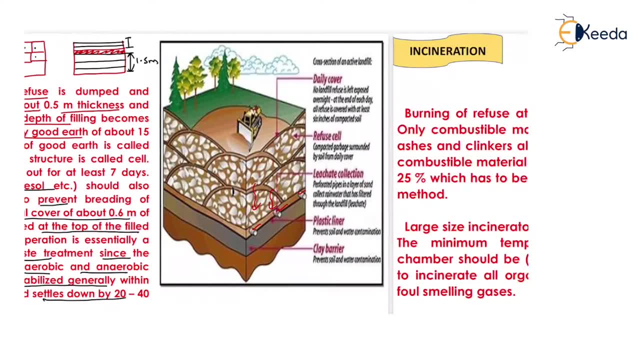 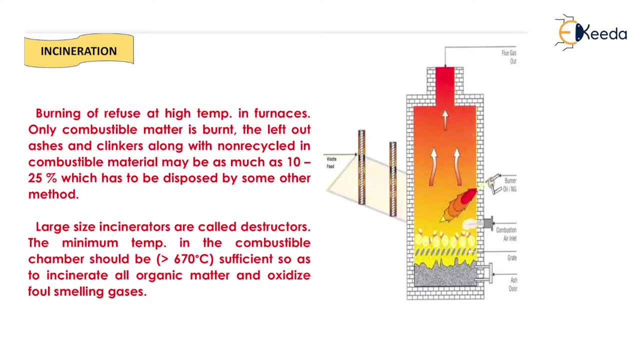 filling process is done or the decomposition process is completely done within a period of 2 to 12 months. that is the sanitary land filling. okay, now the next method is the incineration method. now in incineration we will burn all the combustible matter in the incinerators at a very 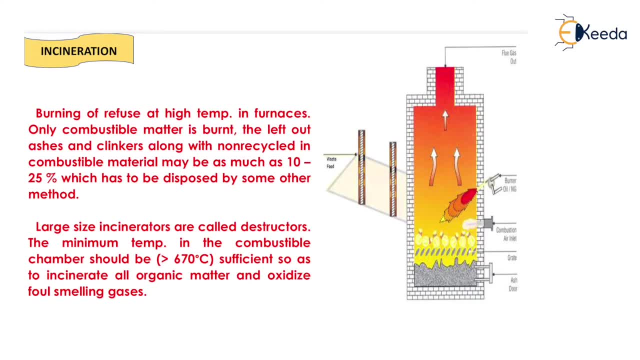 high temperature and all the incombustible material will left out in the form of ashes, which is to be disposed by some other methods. okay now, burning of refuse at high temperature in furnaces is known as incineration. only combustible matter is burnt and the left out ashes and 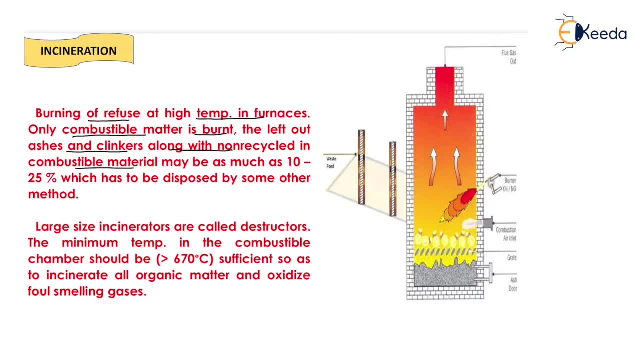 clinkers, along with non-recycled incombustible material, may be as much as 10 to 25 percent, which has to be disposed of by some other method. we had already discussed it that only combustible matter will be burnt and all the incombustible matter will be remained in that. 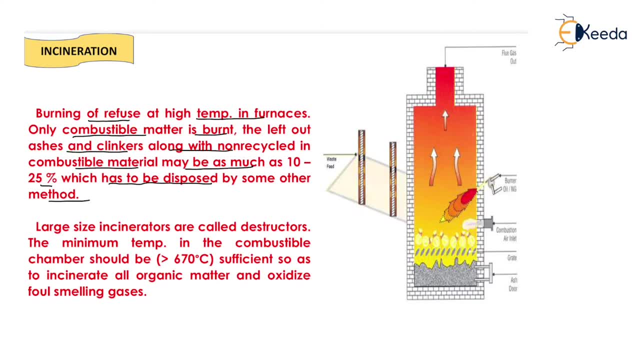 incinerator as a ashes or in the other means such as clinkers etc. now we had to dispose that ashes and clinker by some other means, by sanitary land filling or by composting method. clear. now large size incinerators are called destructors. the minimum temperature in 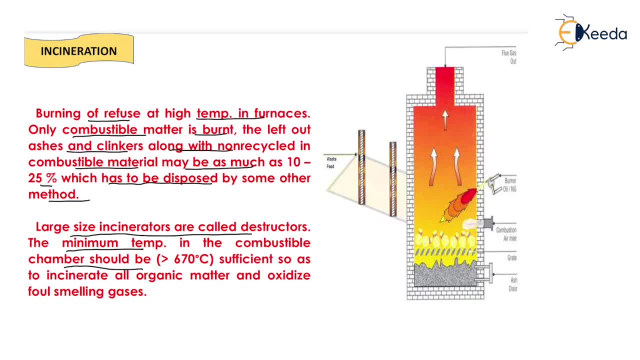 the combustible chamber should be greater than 670 degree celsius, which is very high temperature, so as to incinerate all organic matter and oxidize foul smelling gases. why we kept this much high temperature? to incinerate all the organic matter as well as oxidize. 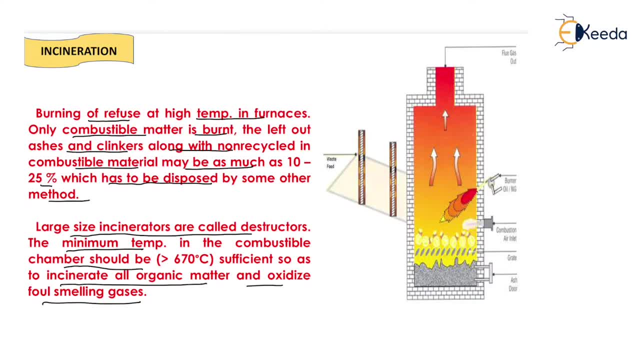 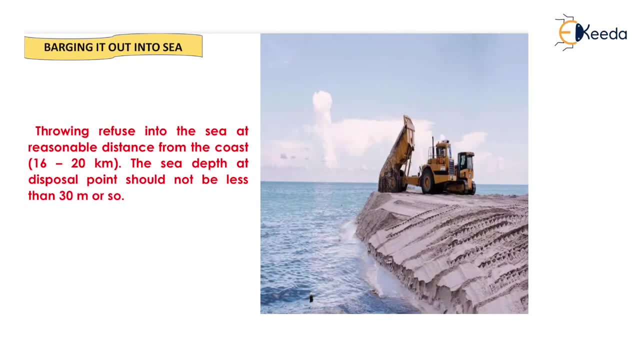 foul smelling gases. that will be the incineration process now. the next process will be the bargain it out into c. now, in this method, we will dispose all the refuse into the sea from a distance of 16 to 20 kilometer from the coastal areas and at that place the minimum depth of c 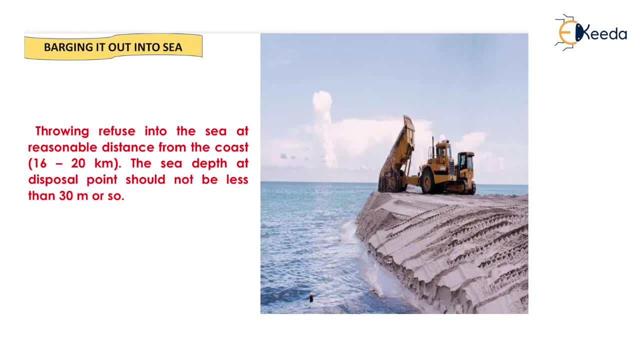 must be 30 meter or so, otherwise we need to move to some more distance. where the depth is greater than 30 meter, we need to dispose that refuse to that sea water. okay now, throwing refuse into the sea at a reasonable distance from the coast, that is, 16 to 20 kilometer, is known as bargain it out into c. now the sea depth at the disposal point. 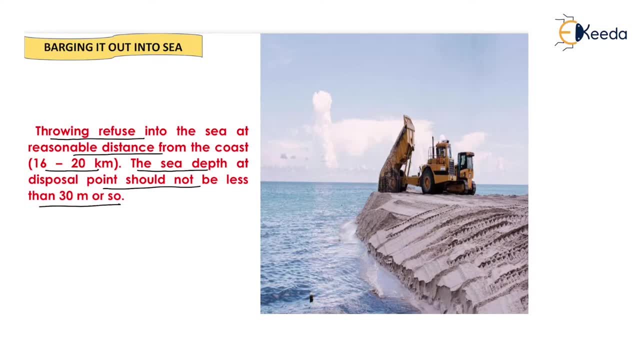 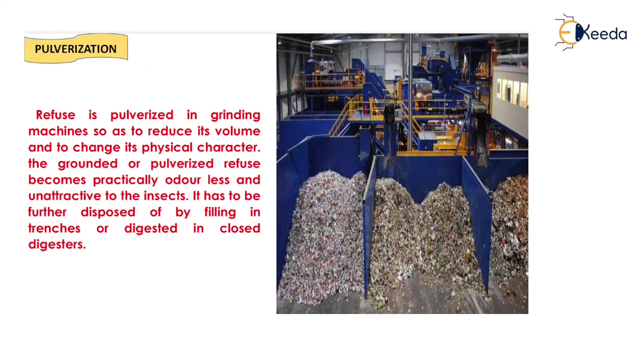 should not be less than 30 meter or so, otherwise all the waste will come with the waves on the coast only. okay, that's why we need to dispose that refuse or that waste where the sea depth is greater than 30 meter. that is the bargain: it out into c clear now. the next method is pulverization refuse. 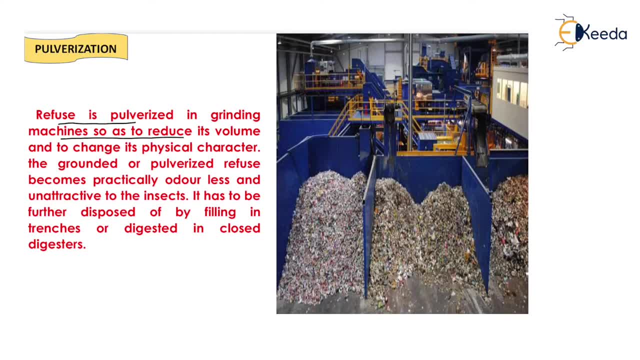 is pulverized in grinding machines so as to reduce its volume and to change its physical character. why we generate to the pulverization? to reduce the volume of the refuse as well as to change its physical character. now the grounded or pulverized refuse becomes practically odorless. 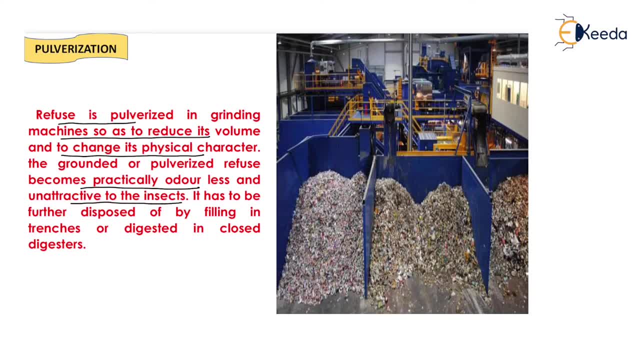 and unattractive to the insect. it has to be further disposed off by filling in trenches or digested in closed digester. it means that after the pulverization process we need to treat that refuse by some other means, such as by sanitary land filling or by 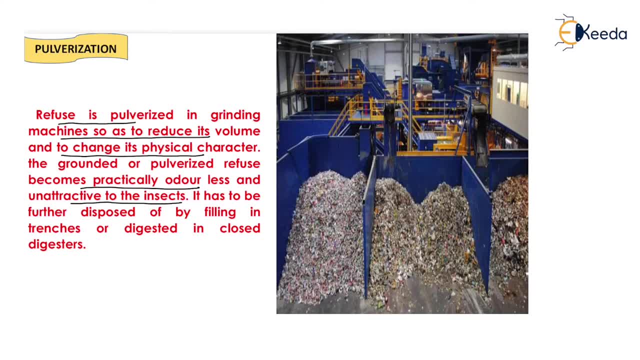 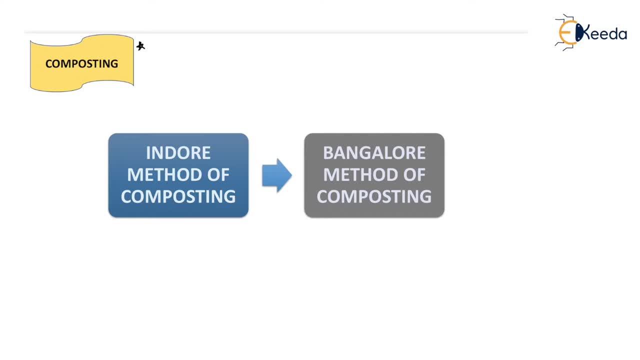 closed digesters. we need to treat that refuse. okay, now, that is the pulverization method. now we will move to the next important topic, that is the composting method of disposal. now, that is the one of the most important method of disposal of composting, that is the indore method of composting. now we have defined the composting method in two. 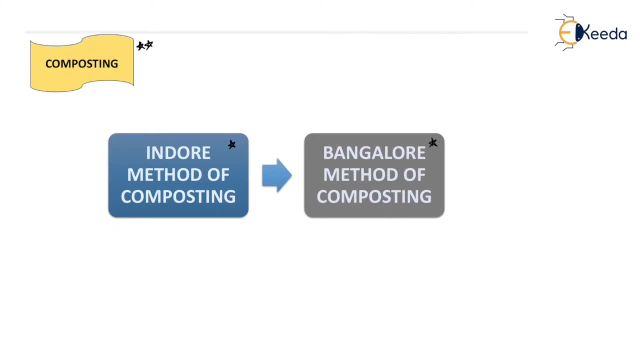 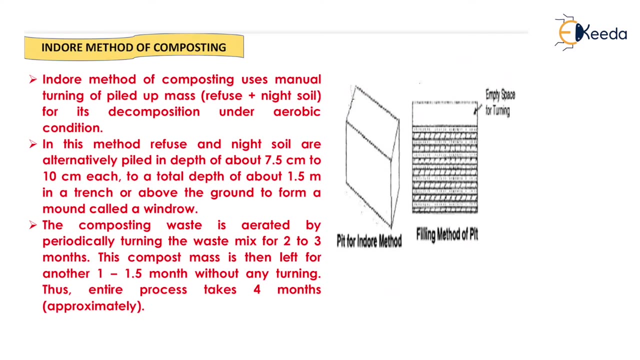 parts, that is, the indore method of composting and the bangalore method of composting. now we will see, one by one, each and every method in detail. okay, starting with the indoor method of composting. now, in indoor method of composting, we will fill the trench by the alternative layers of refuse. 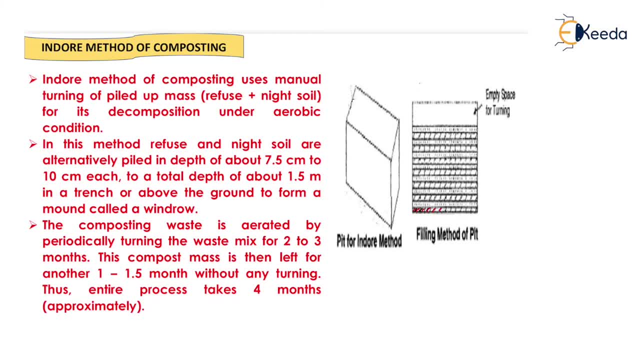 and night soil. we will keep in one layer refuse and in another layer the night. that is the human waste- okay, human excreta or human solid waste- clear now. in another layer, refuse will be there and above that night soil will be there. similarly, another layer refuse will. 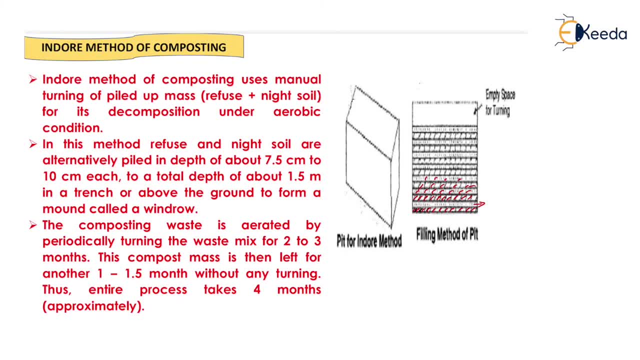 be there and night soil will be there now, after filling the complete trench of height of 1.5 meter. now what we will do? we will just left this mass as it is and by periodically turning that mass for two to three months, we will keep that mass aerated for the two to three months now. 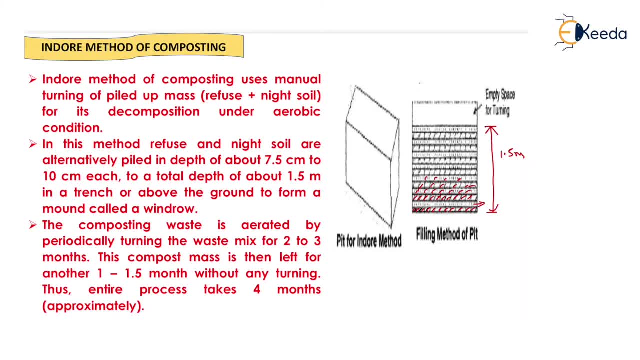 during this process of manual turning of the piled up mass, we will keep the aeration process in that mass. due to this aeration process, the aerobic bacteria will do the decomposition of the organic matter and all the organic matter will be decomposed after four to four point five- months. 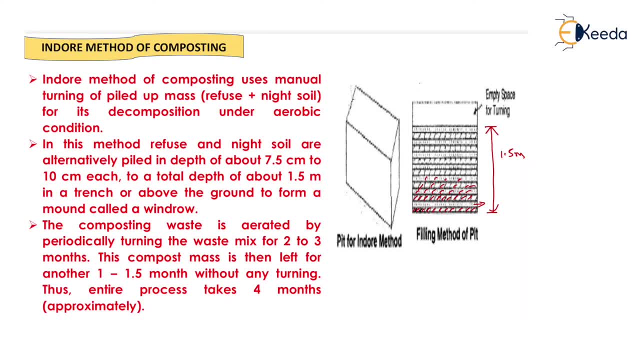 okay, so after two to three months of manual turning- what we will generally do- we will left that piled up mass for the one to one point five months without any turning. now, after one to one point five months, all the organic matter will decompose completely. now what is the problem with? 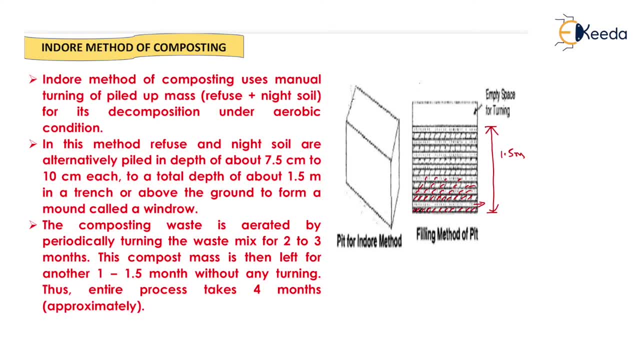 this method. why the municipal department will not use this method nowadays? because during the turning of the piled up mass, all the waste will spread into that area and it will cause pollution in that area. that's why indoor method of composting is outdated nowadays. okay, now in indoor method of composting uses manual turning of piled up mass. that is refuse. 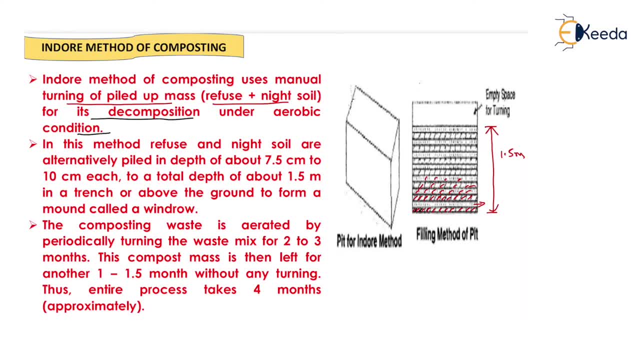 plus night soil for its decomposition under aerobic condition. we had discussed it now. in this method, refuse and night soil are alternatively piled in depth of about 7.5 centimeter to 10 centimeter each, to a total depth of 1.5 meter in a trench or above the ground to form a mound called windrow. 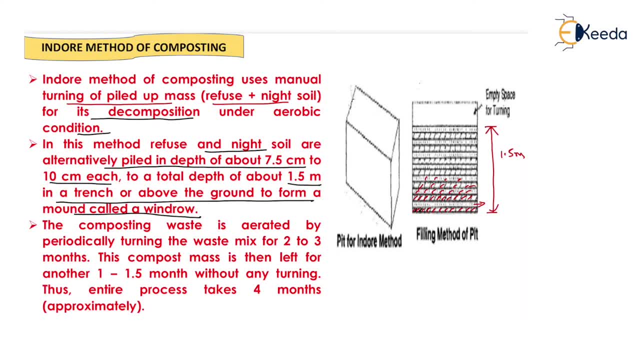 in land filling we call the small unit as cell. here the small unit is known as a cell as windrow. now the composting waste is aerated by periodically turning the waste mix for two to three months. we had already discussed it, that initial phase we need to turn the waste mix for 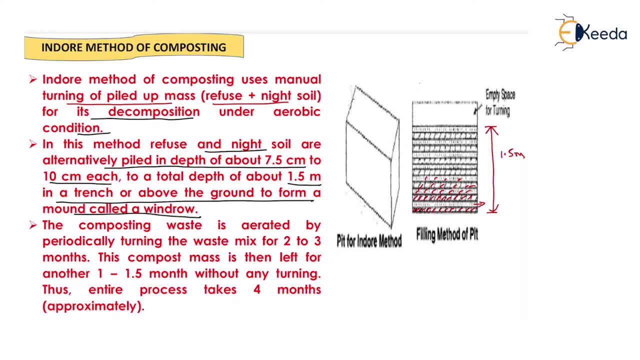 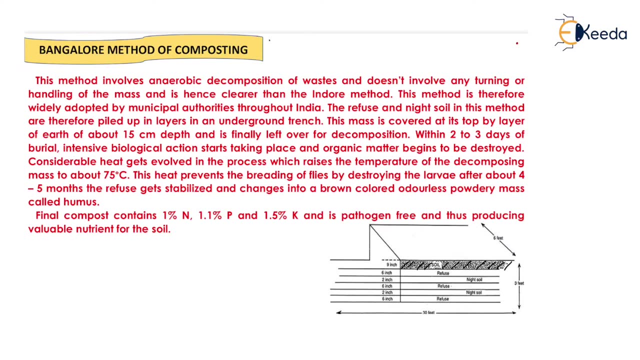 two to three months, okay now. this compost mass is then left for another one to one point five months, without any turning. thus entire process takes four months for the complete decomposition of the organic method. that is the indoor method of composting. now the next method of composting is. 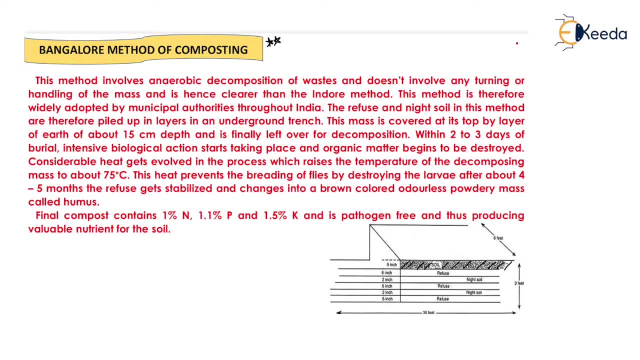 the bangalore method of composting. now, the next method of composting is the bangalore method of composting. now, in bangalore method of composting we will make the windrow as one layer of refuse, another layer of night. so in one layer of refuse, another layer of night. so in one layer of refuse. 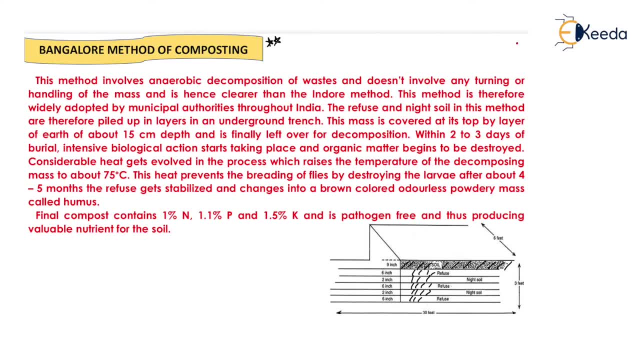 and another layer of night soil. similar to the indoor method of composting, but the difference is that in indoor method the process is aerobic, but in bangalore method the process is completely anaerobic. now what, how this anaerobic condition will arise here? just listen to me, okay. 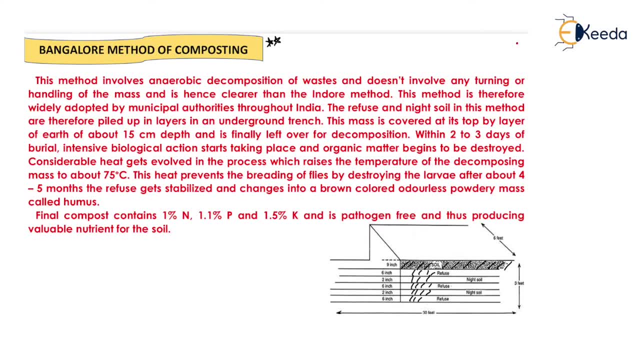 now, when the complete area is filled by the refuse and night soil, we will provide at the top the soil layer or the earth layer, of thickness 15 centimeter to 20 centimeter. now, this soil layer will restrict the entry of air from the atmosphere to the refuse or night soil, due to which anaerobic 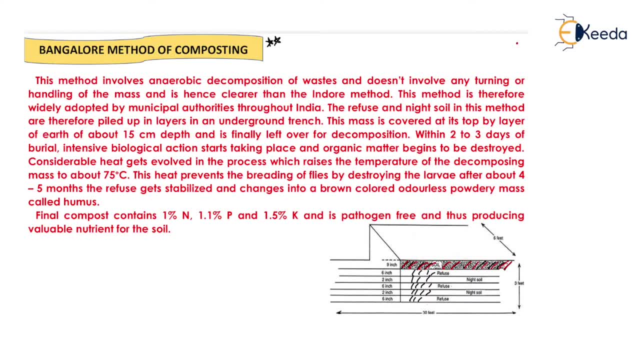 condition will arise into that piled up mass and, due to this, anaerobic bacterias, all the organic matter will die out and the organic matter will die out and the organic matter will die out and the decomposed due to anaerobic bacteria, and the whole process will take around four to 4.5 months. 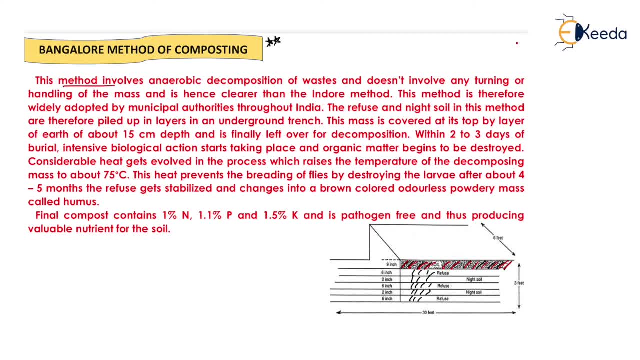 okay now. this method involves anaerobic decomposition of waste and does not involve and does not involve any turning or handling of the mass. hence it is clearer than the indor method. hence it is clearer than the indor method. that's why all the municipal department nowadays used 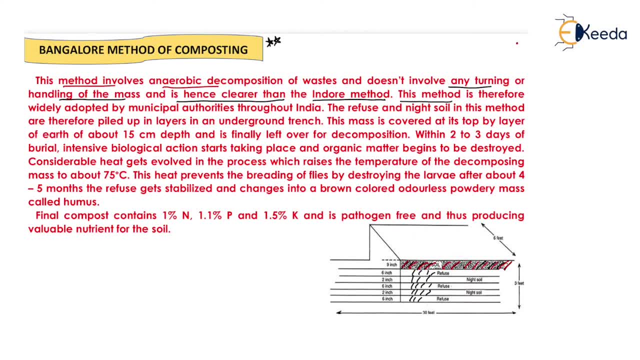 bangalore method of composting. this method is therefore widely adopted by the municipal. that's why all the municipal department nowadays used bangalore method of composting. this method is therefore widely adopted by the municipal它's right Hoje 1800 algún creator s Кор? method of composting. by the municipal lieder. the following method is an eight moving will be adopted in bangalore. the trouble yet. this method is therefore widely adopted by the municipal lieder, our particulate property. the material of decomposition is thi niâong y regular Kook bin thyor et al gbihai he iswater秋af Nicolas Hari thao". 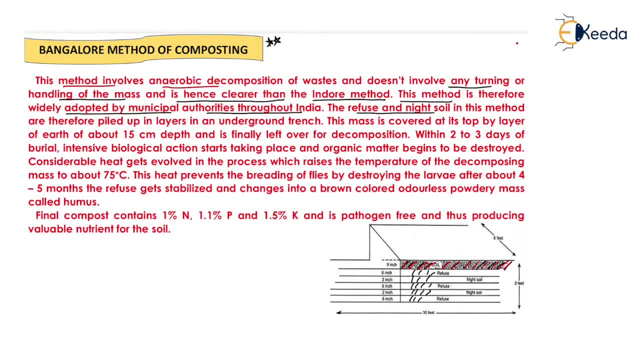 authorities throughout India. The refuse and night soil in this method are therefore piled up in layers in an underground trench. This mass is covered at its top by a layer of earth about 15 cm depth and is finally left over for the decomposition Within 2-3 days of. 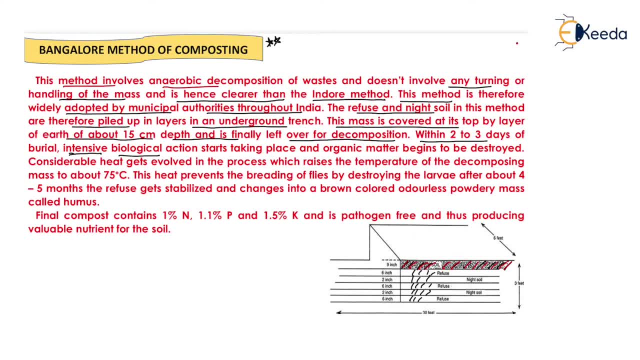 the process, intensive biological action starts taking place and organic matter begins to be destroyed Due to this decomposition. considerable heats get evolved in the process, which raises the temperature of the decomposing mass to about 75 degrees Celsius. Now this high temperature will indicate that the decomposition is started and, slowly and slowly, the temperature will 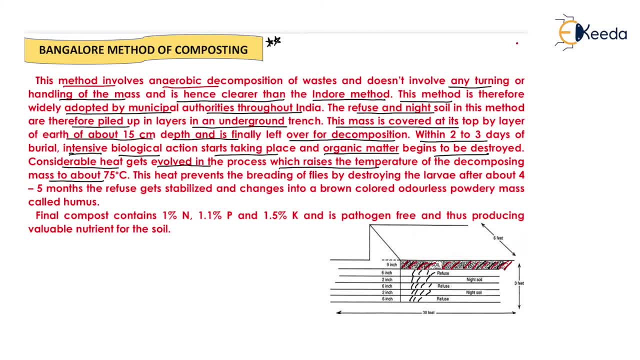 decrease and the whole process, or the decomposition process, is completely done slowly and slowly. Now, this heat prevents the breeding of flies by destroying their larvae. After about 4-5 months the refuse gets stabilized and changes into a brown colored odorless. 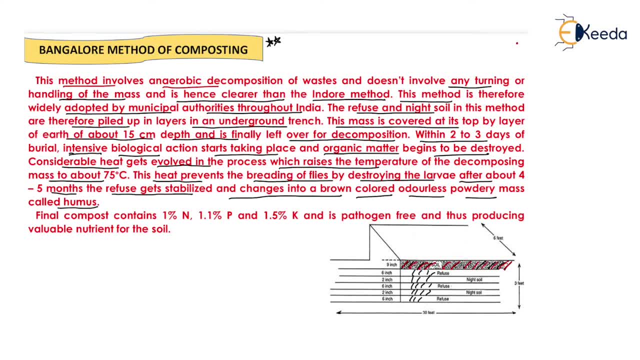 So all the organic matter will be converted into humus, which will contain 1% nitrogen, 1.1% phosphorus, 1.5% potassium, and is pathogen free and thus producing valuable nutrients for the soil. That is all about the composting method. We had discussed the fundamental definition. 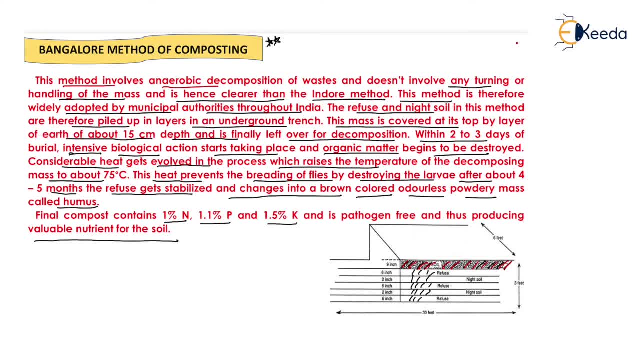 as well as the method of disposal of solid waste management. That is all about this topic. Thank you very much for watching this video. Thank you very much, students.